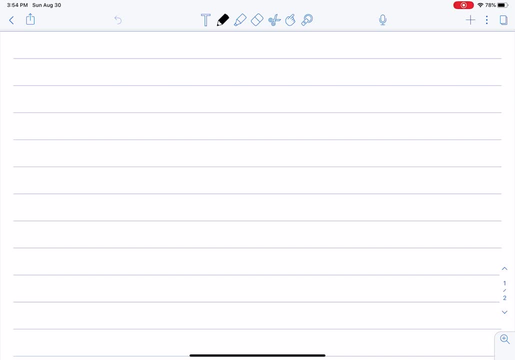 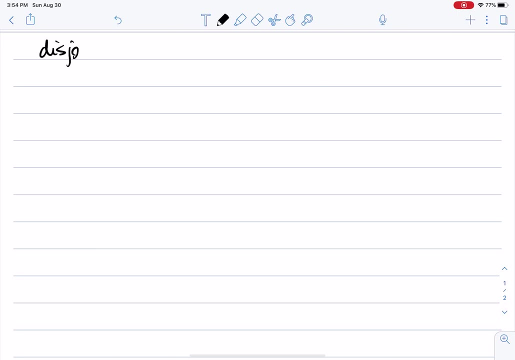 Another representation of disjoint sets is what we call disjoint set forests. So disjoint set forests. So a forest is just a set of trees. So if we think about it like that, then remember that we have a set of disjoint sets. 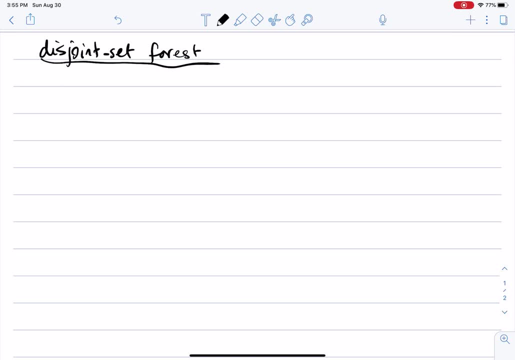 We're going to represent each individual set as a tree. So imagine that I have two sets. One is, let's say, A, C, E, G, H, J, D. Okay, whatever, This is a set. There's no order on it. 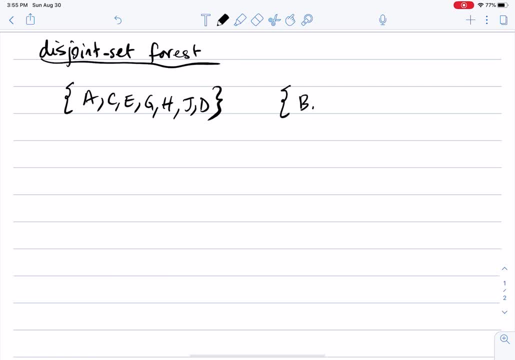 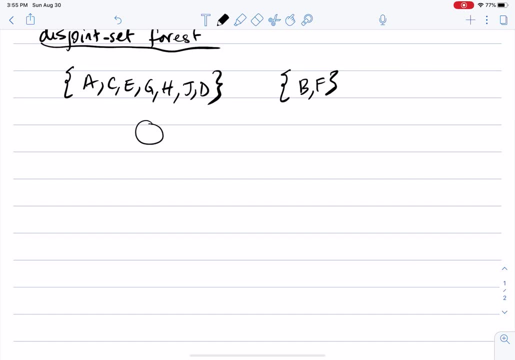 Okay, and suppose I have another set that is B and F. So one way to represent each set is as a tree. So imagine that this is a tree And C here. I have, E I have, let's say, J here. 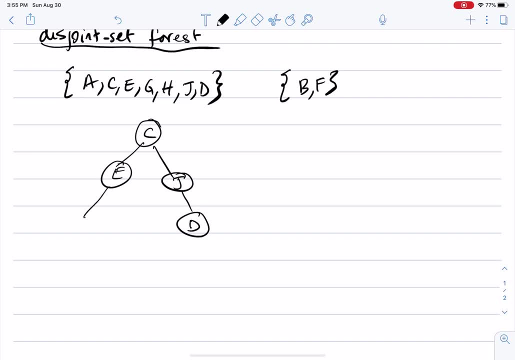 And I have D. I have imagine that I have three children here, G, A, and I believe I got all the letters now. Now, each node is going to point, it's going to have a pointer to its parent. 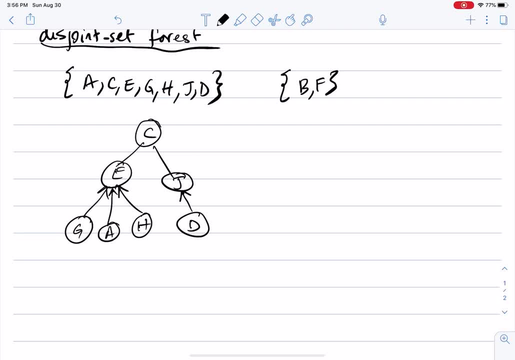 Okay, so each one of them is going to have a pointer to the parent. This is the information we're going to store. Of course, the root is named Nell. Okay, the parent of the root is Nell, So this is a tree structure that represents that set. 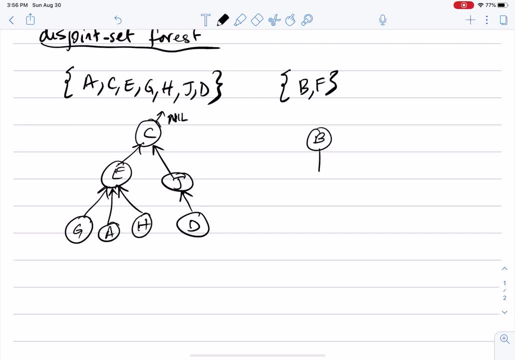 And for BF, for example, it could be BF. Okay, so this is. So. if you look at this, here we have a set of two trees. This is what we call a forest. Okay, so we have two trees like this. 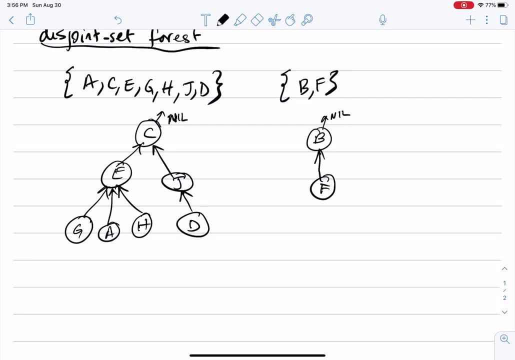 And we always have. when we talk about a set, we always have a pointer to the root of that tree. Okay, so I can have. I have a pointer to this and a pointer to this. If we have this structure now, so what about making set? 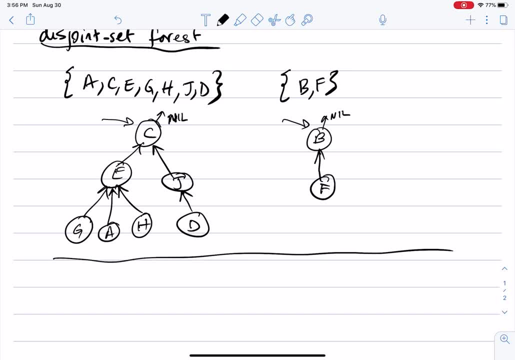 If we look at this, Notice that the trees, by the way, are not necessarily binary. And if I want to do, make set. Okay, make set set of X. All we need to do is just something like this: right. 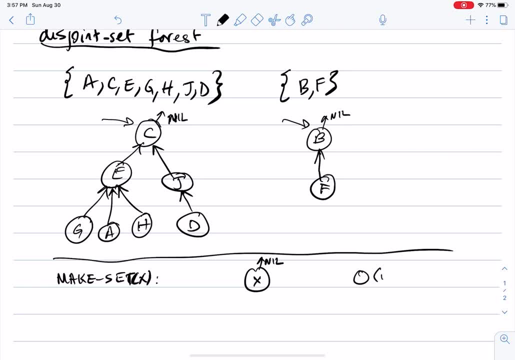 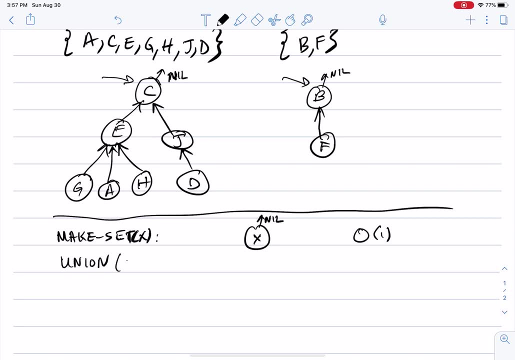 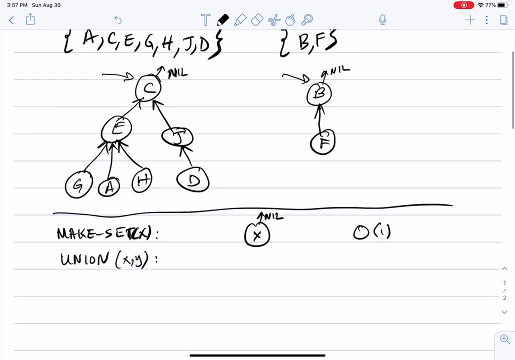 It's a tree with a single node, whose parent is Nell. It's O of one operation. What about phi? sorry, union of X and Y. Okay, and suppose X and Y here are the roots of the tree. Well, in this case, if I look at the top two trees here, the BF and the other one, 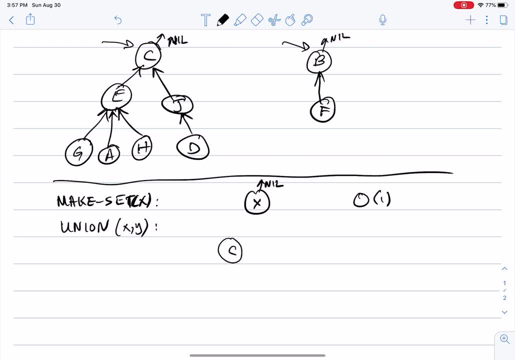 one way to do the union is so. I have C here, E, G, D. I'm not drawing the arrows here, but the arrows are pointing up G, A, H And I have this tree here, BF. 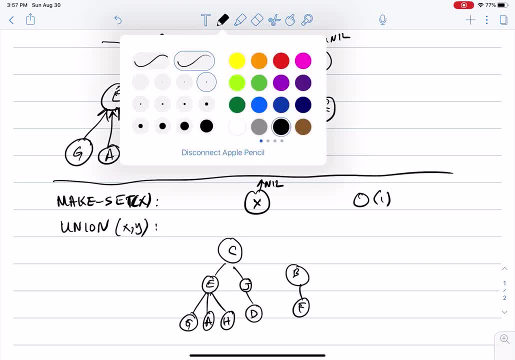 And the way we do the union is. now I can say that the parent of B is C, The parent of B is C here. okay, So this is how we do the union, because now I have pointers to the roots of the two trees. 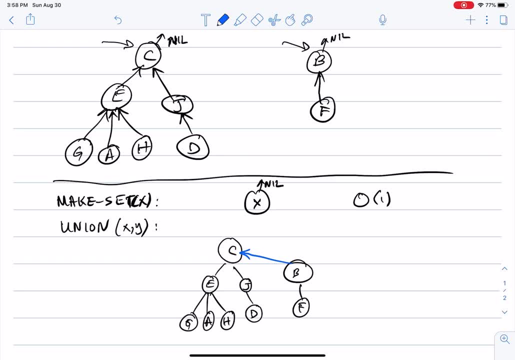 Okay, so now I have pointers to the roots of the two trees. I look at the space. The smaller of the two trees the smaller in terms of the number of nodes. So this tree has two nodes in it. This tree has seven nodes in it. 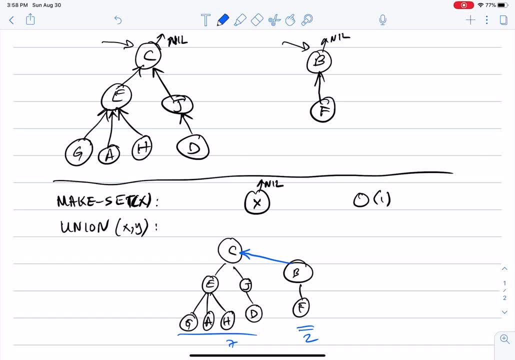 I will do the union by making the root, the parent of the root of the smaller of the two trees- point to the parent of the larger tree. okay, So if you think about this, here, all I'm doing is make the parent of the root of the smaller tree. 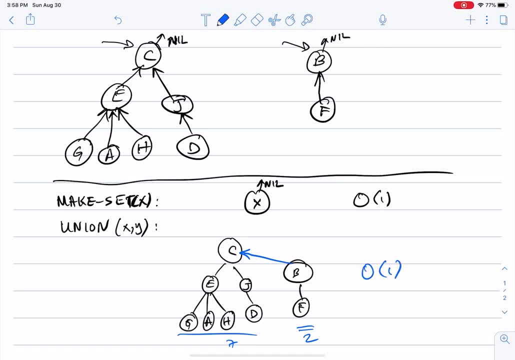 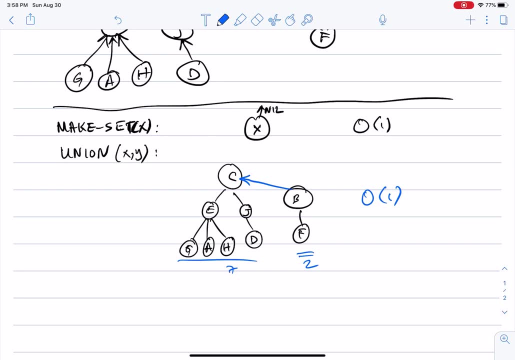 point to the root of the larger tree. It is also O of one operation. okay, Now, in the linked list representation the union was the costly one. Make set and find were the easy ones or the cheap ones Here. in this case, make set and union are the cheap ones. 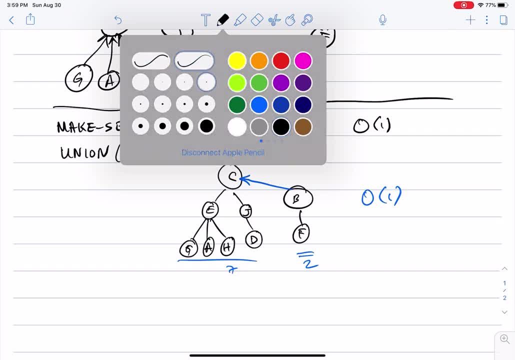 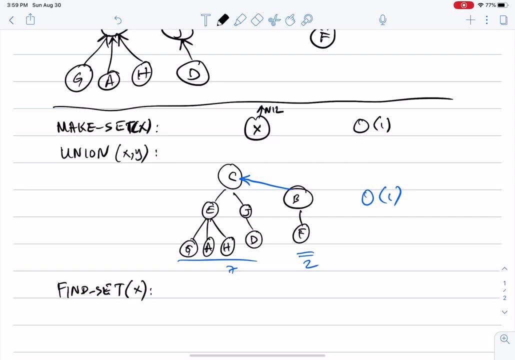 Each one of them is O of one operations. But what about find set? Find set of X. So suppose I say here, in this case, find set, Set of G. So how do we find set of G? 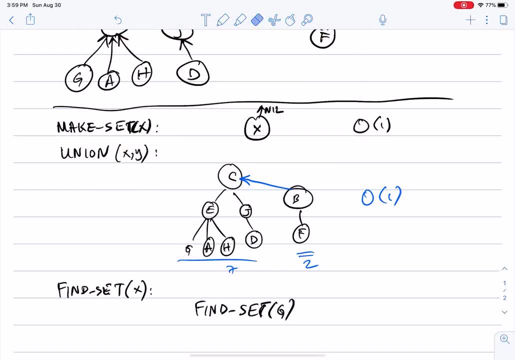 Again, remember that in all these cases- I'm saying I'm giving you a pointer, I'm giving you a pointer to that element that I'm asking you to find- The only thing you need to do is look at the parent and the parent. 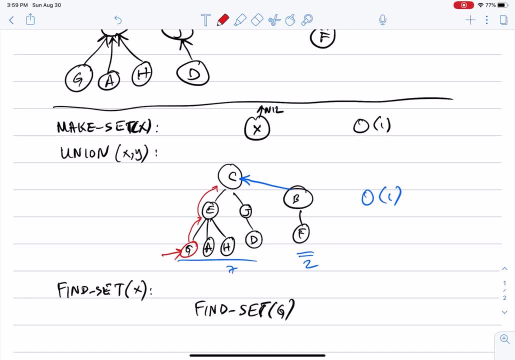 You keep going up until you get to the root of the tree and you say: this belongs to set C. okay, The set whose representative is C. And if you think about this now, that in the worst case, the running time of this algorithm of finding set 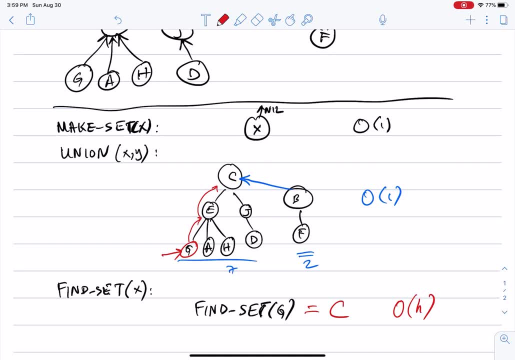 is on the order of the height of the tree. okay, So if the tree is very, very high, this operation is going to be expensive. If the tree is not very high, it's going to be cheaper. Now the question is: given the way we do the union, 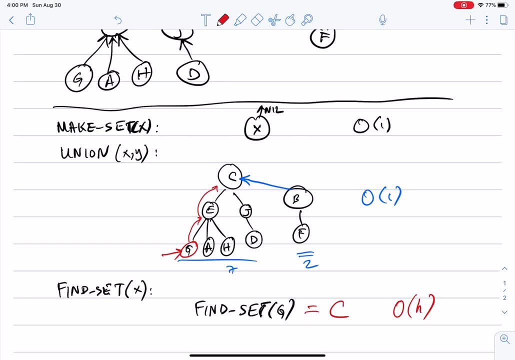 and, given the way we do this, make set what is the height of the tree. okay, Even though the tree is not binary, it seems that we could add any trees in any order we want. I want to remind you that the three applications, for example, 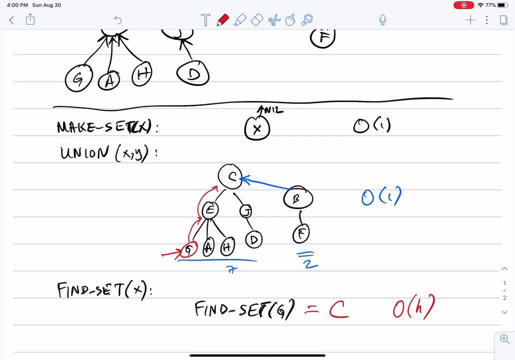 I illustrated at the beginning: equivalence classes, minimum spanning tree and connected components. all of them started with in operations of make set. in operations of make set, each of which made a set of one element in it. Then the union operations applied on that. 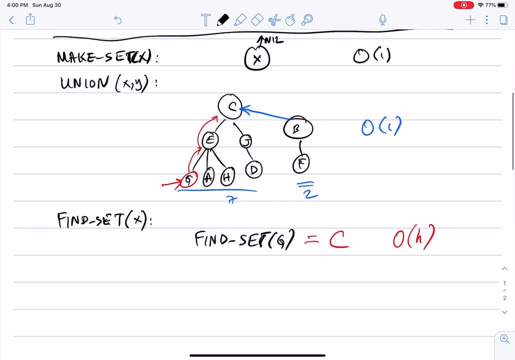 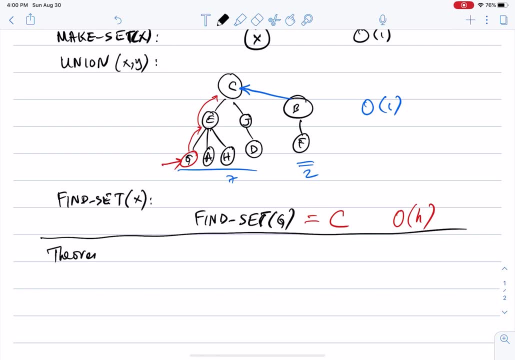 So I want- I want to now talk about the height of the tree in such a scenario here. okay, So I want to basically say that I want to talk about a theorem here that let T- let T be a tree. 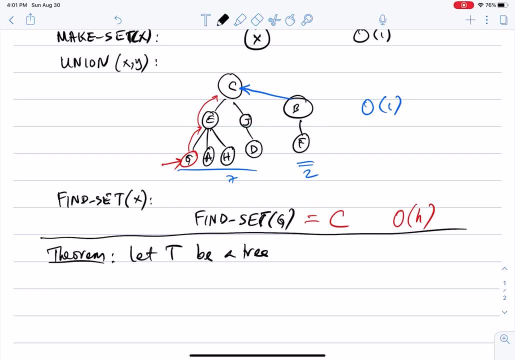 representing a set of a tree, representing a set, A set Of n elements. A set of n elements, But not any tree. It was constructed. So a set of n elements that was constructed, A set of n elements that was constructed. 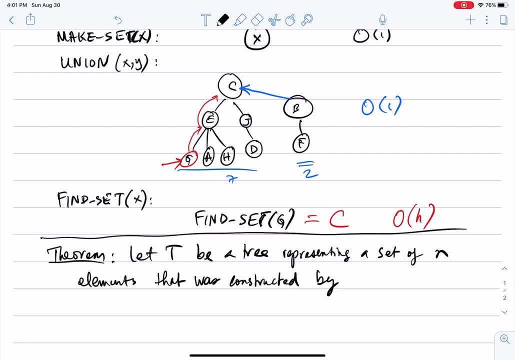 by n calls by n calls to make set Okay. So by n calls by n calls by n calls by Quel denotes unit? by n, then made n in singletons and then followed by calls to Union. 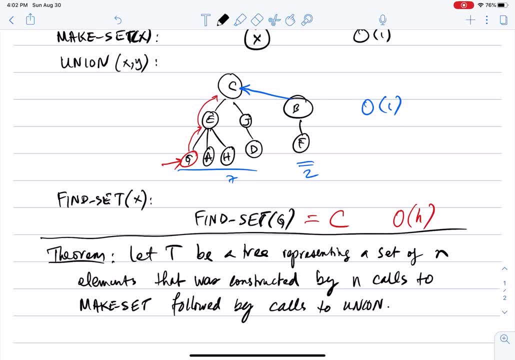 okay, So let tree T be a tree that has n nodes in it. That tree was built again because of the way the algorithms and the applications of these data structures are, the way it was built in operations of make set, and then after that we call the union again, n minus one times, such that 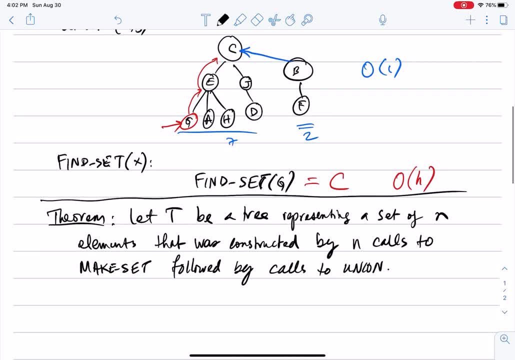 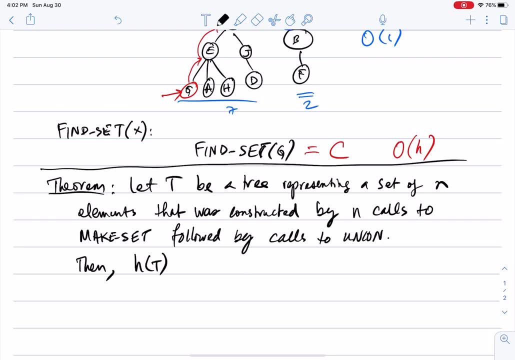 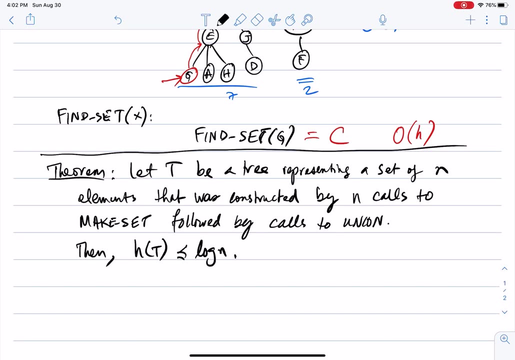 we got a tree that has, that has n elements in it, then i would say: then the claim is that the height of the tree h of t is at most log n. okay, so this is the theorem that if we do the operations in the following way: first we created n singletons and then we did the union operations on it, 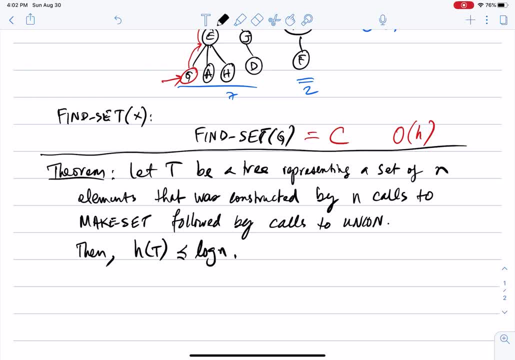 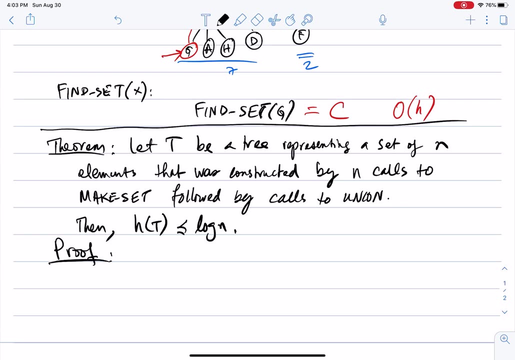 the height of the resulting tree cannot be worse than log n. okay, because keep in mind again the way the union works: it always merges the smaller of the two trees to the larger of the of the trees. okay, and the proof is actually very simple and is always, on these cases, by induction on the height. 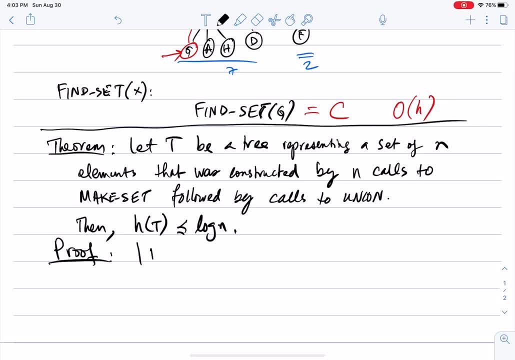 of the tree. okay, so i will use notation that the cardinality of t is, at most, log n minus one times t is the number of nodes in t and t, and again i'm using h of t as the height of t. okay, what do i want to show here? i want to show: 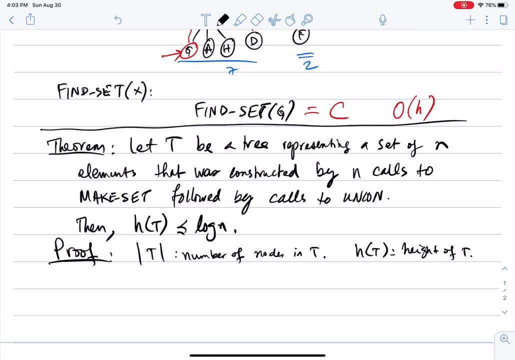 that the tree t again, that's built in such a in such a way satisfies t. the size of t is greater than or equal to two of h. okay, this is what i want to show. we want to show why is this? why does this prove what we are interested in? because, again, take the log of. 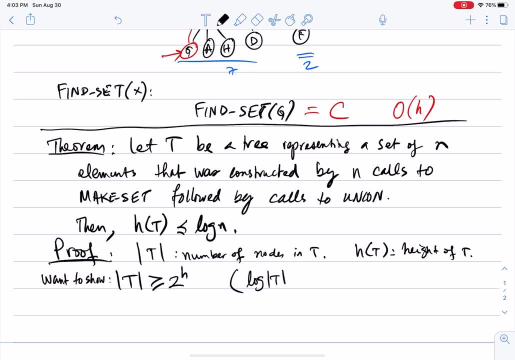 both sides, you will get the log of the size of t greater than or equal to h. okay, so i want to basically show that if we build a tree with n nodes, by first calling make set n times and then doing the union on it to build a tree with n elements in it or n nodes in it, then the height 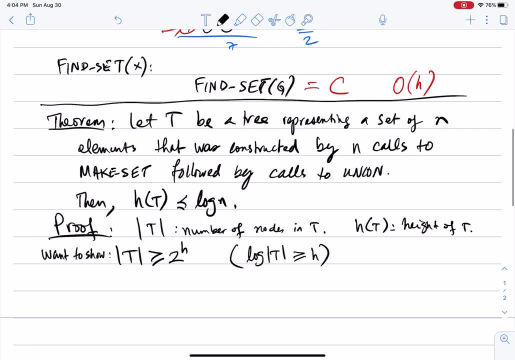 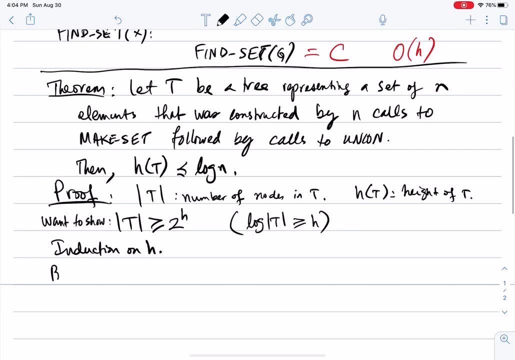 of that tree cannot exceed log n. okay, and the proof again is induction on h. okay, so the base case, the base case when h is zero we have, the size of the tree is one. it has one element in it and one is greater than or equal to two to the zero, two to the h right. so 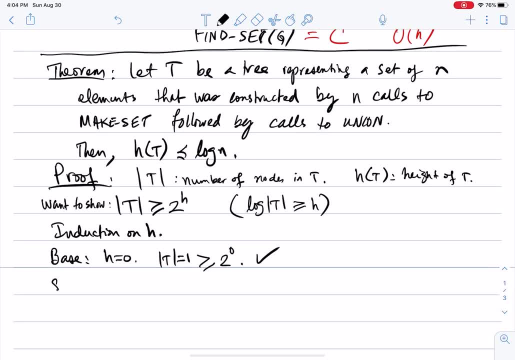 the base case holds. okay, now we want to do the inductive step, and the way i will do it is as follows. again, it's by by strong induction or induction of the tree, and it's one element in it and one is greater than or equal to two. two to the. 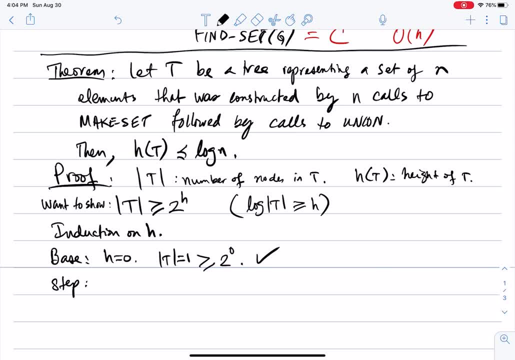 this case by structural induction. so we need to think about assuming something about the trees that we are going to use to build the treaty here. okay, so now assume that for any, for any tree is that if the height of s is smaller than or equal to h, then 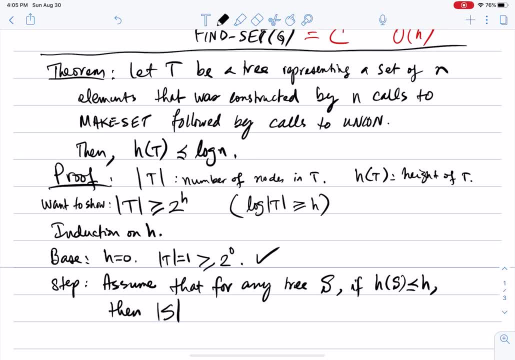 the number of nodes in h is at least 2 to the h of s. okay, this, this, all of this here. this is the inductive hypothesis. okay, this is the inductive hypothesis i am saying. i want to know, prove something on trees whose height is h plus one. so i will assume that for any tree whose 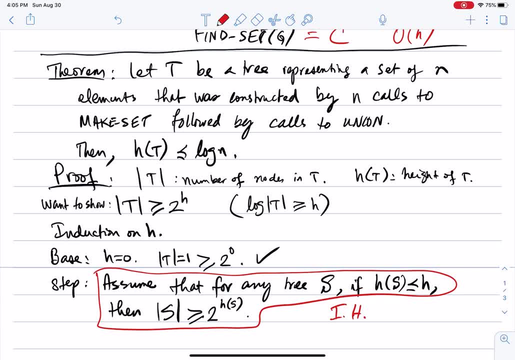 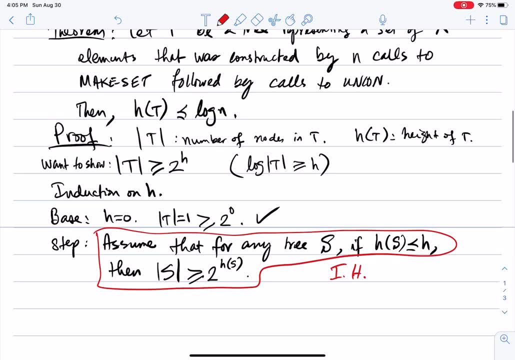 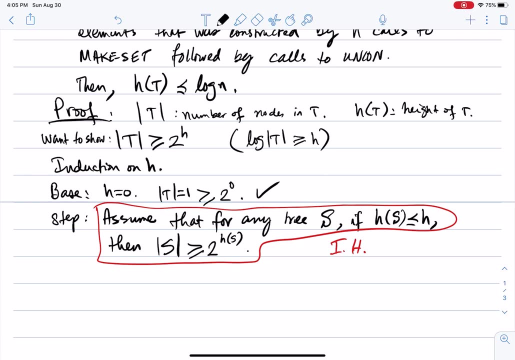 height is at, is h or smaller than h, then the number of nodes in that tree is at least two to the h of that, to the height of that tree. okay, so this is the inductive hypothesis. now and now let's look at t. that let's assume. now let t. t is a tree, is the first tree, the first tree created. 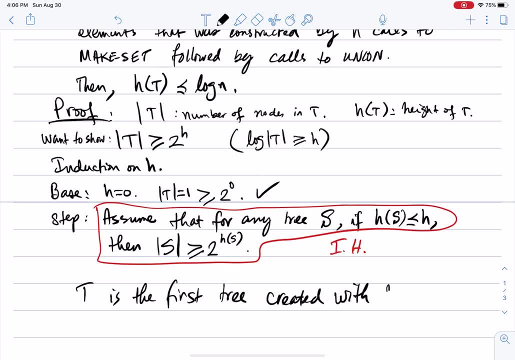 with height h plus one. okay, what does this mean? remember that we have a set a, a list of union operations. so the first union created a tree of size two. the second union could have created a tree of size of height three, and so on. what i'm saying is that, in by inductive hypothesis, i am assuming- 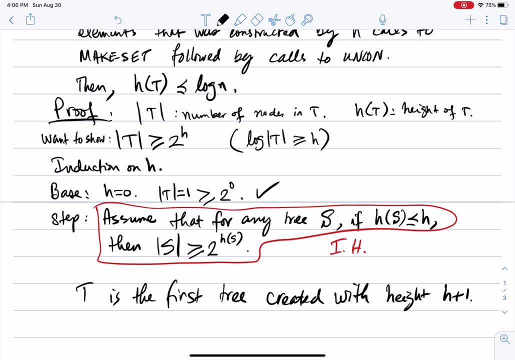 something about all trees whose height is up to h. now i'm saying let t be the very first tree we see during the algorithm whose height is h plus one. okay, so tree is the first height, the first tree whose height is h plus one, the first tree whose height is h plus one. 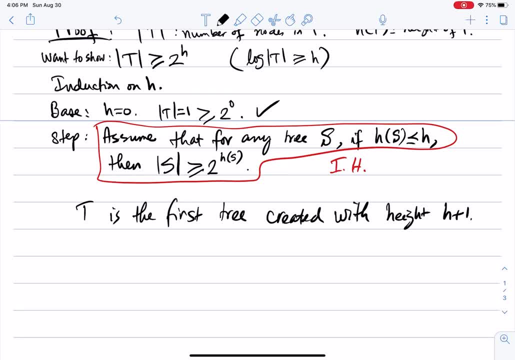 the first tree whose height is h plus one, then the tree t must have been built like this. the tree t is as follows: it has two components here: t1, t1, and we had t2 and the root of t2 pointed to the root of t1. this whole tree is t, okay, this. 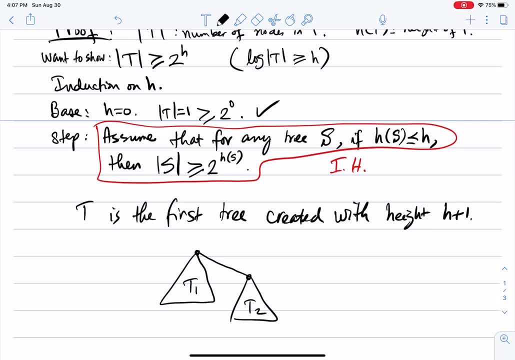 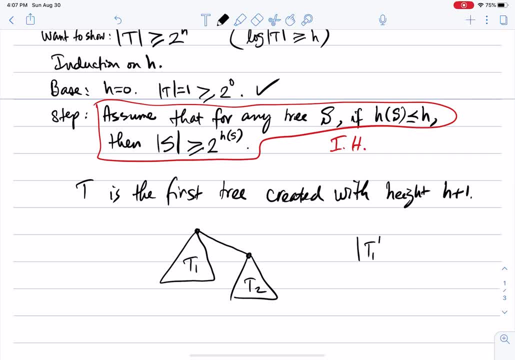 the, the union, that the number of nodes in t1 is at least the number of nodes of t2, because we merge the smaller of the two trees with the larger one. but in addition i know that the height of this full tree here okay. so the height of the tree t h of t is h plus one. right now we know that t, the. 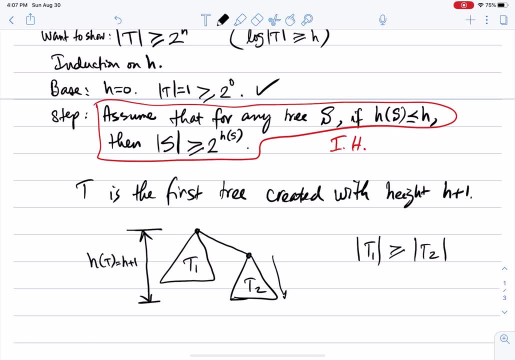 height of t2 is h here. why is it h? because t1 is the height of t1 is at is at most h. the height of t1 is at most h here. so the height of t1 is at most h. why is it at most h? because if it was h plus one, then that violates the assumption that 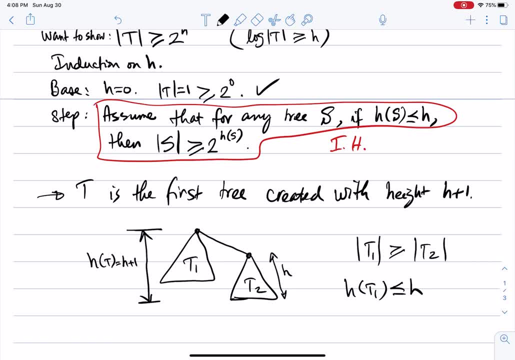 t is the first tree created with with height h plus one. so if the height of t1 is at one most h to make a tree by union with, that will will create a new tree whose root is the root of t1 and whose height is is h plus 1, then I must have added a tree. 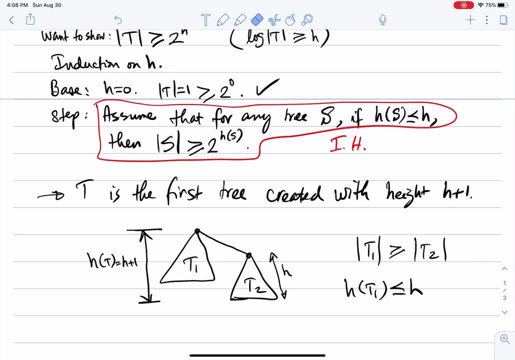 whose height is H and added it to the root, because now the height of T is that H, the height of that tree is this H here plus 1 for this, for this edge here. so this is where we get the h plus 1 the height of T. okay, so we know that the 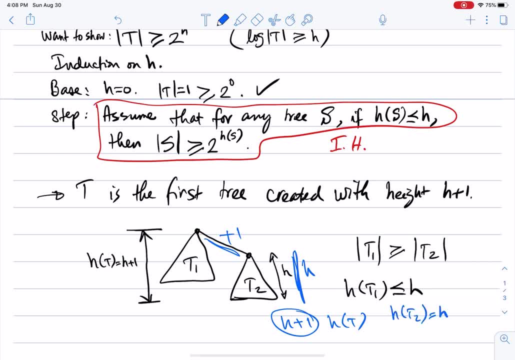 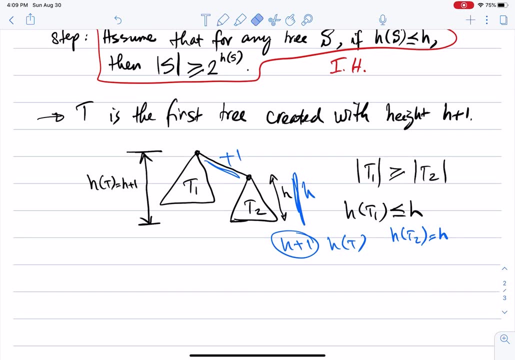 height of T 2 is H. we know the height of T 1 must be at most H, and now the height of T is H plus 1 using this construction. okay, so then we know that by the inductive hypothesis, by the inductive hypothesis, then. 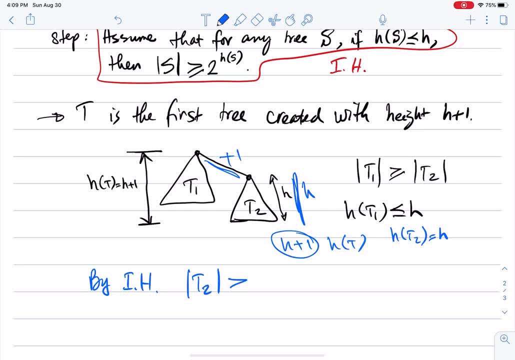 that number of nodes in t2 is at least 2 to the h. okay, because its height is h. now we also know that the number of nodes in t is the number of nodes in t1 plus the number of nodes in t2. we don't create any new nodes here. the root of t2 points. 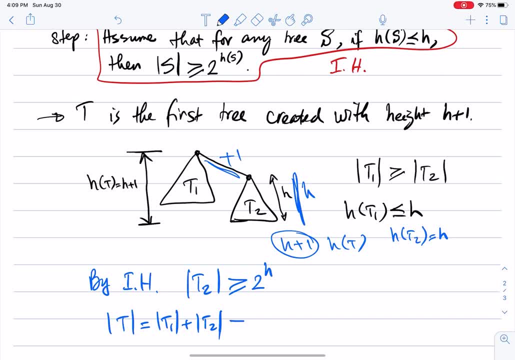 to the t1. so these numbers, we know that, we know that the the number of nodes in t1 is greater than or equal to t2, so these are greater than 2 times right in other words. I mean, if I want to write it so with more clarity here, just so that 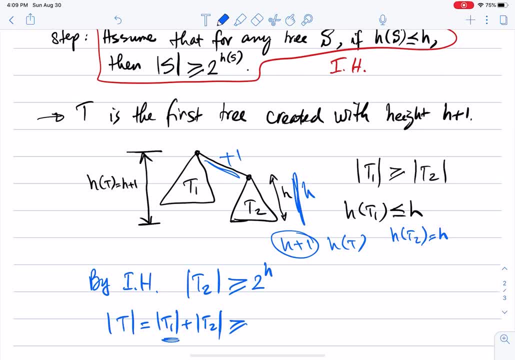 nobody misses it. we know that the size of t1 is greater than or equal to the size of t2 and we know that the size of t2 is greater than or equal to the size of t2 vacuously. and this is 2 and t2 here. 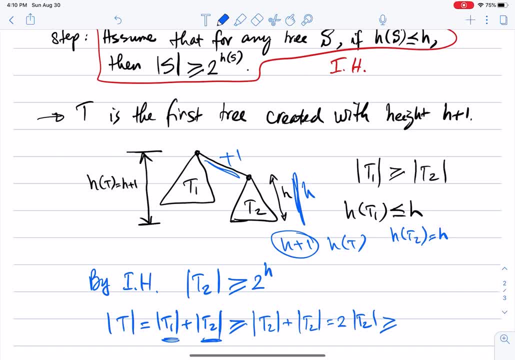 and this 1 is here will be basically now greater than 2 times 2 to the h, which is 2 to the h plus 1. okay, where did i get? the size of t2 is 2 to the h by the inductive hypothesis. so now, what we showed here is that 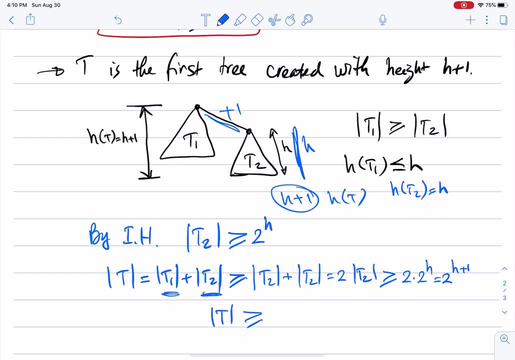 what we showed is that the size of t is greater than or equal to 2 to the h plus 1. so now we have proven that a tree that is built in the in the, with this sequence of operations will have the number of nodes in it is at least 2 to the h of that tree. therefore, the height of the tree is at: